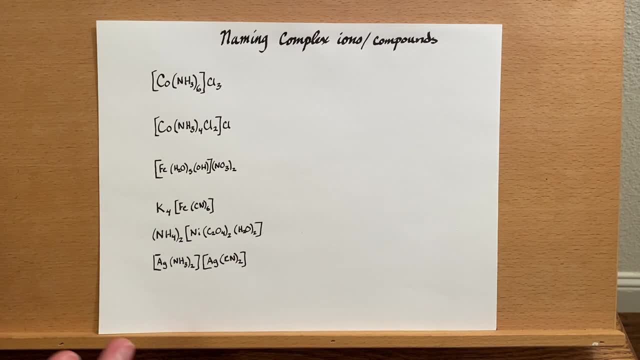 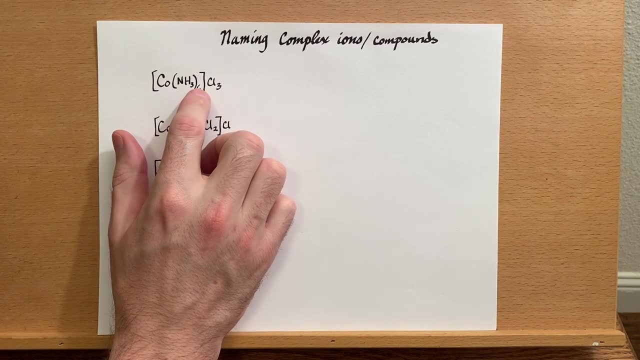 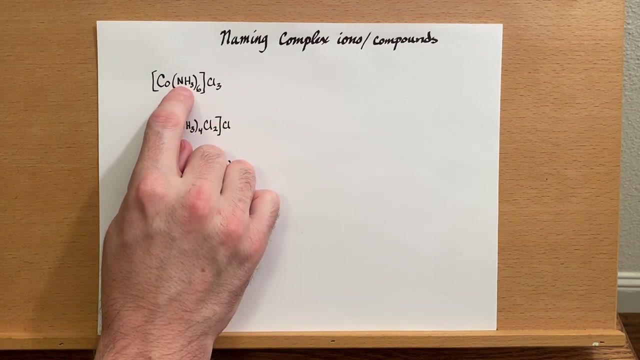 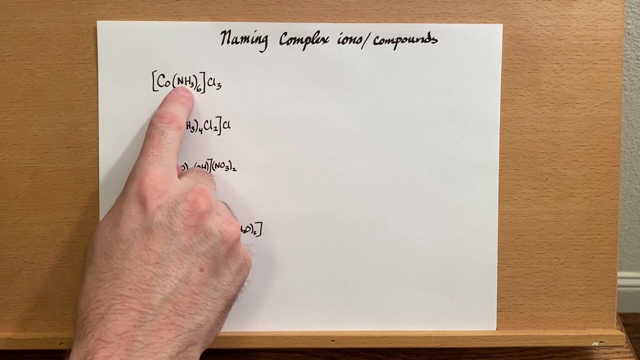 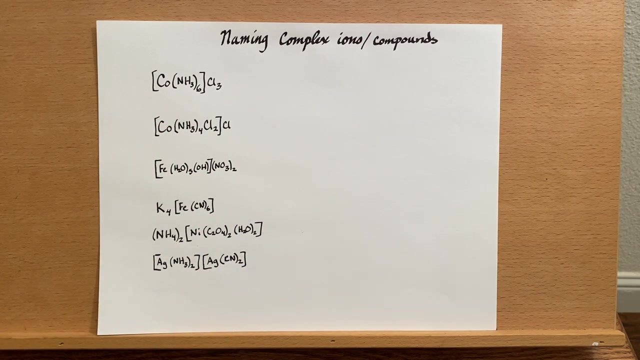 following that. so just keep that in mind and don't forget the original rules that we learned before. so we really just need to know the name of this part now. ligands have their own little names when this is an ammonia group, but when it's bound to a metal we call it amine, and there's six of them. so we say hexamine, cobalt, three. 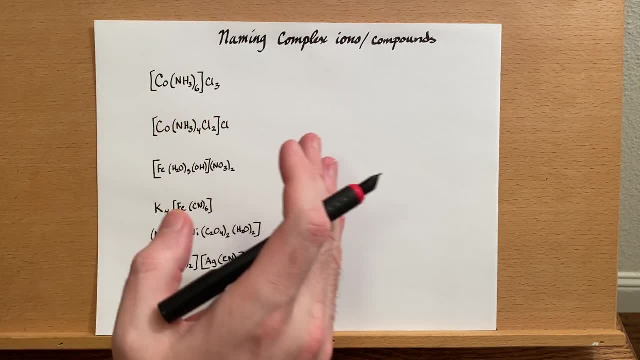 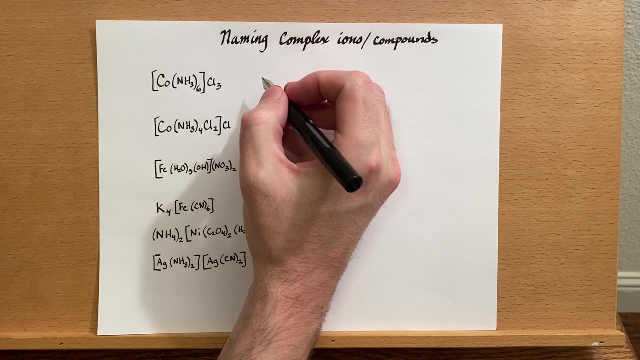 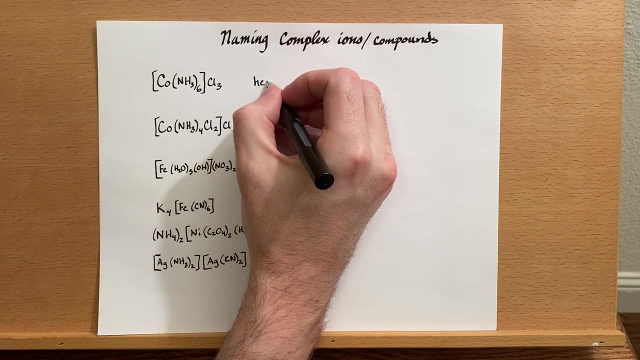 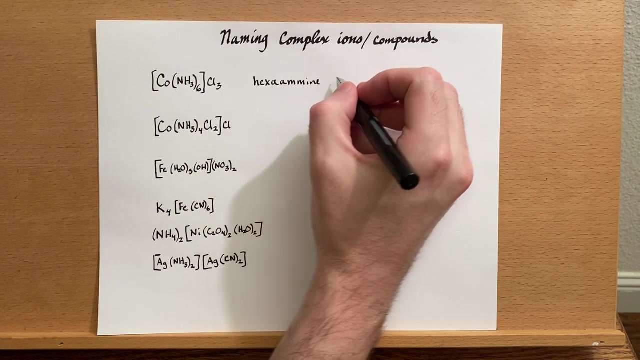 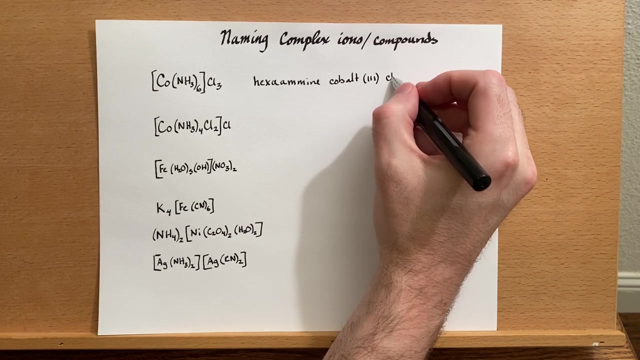 because that's the charge of the cobalt and then chloride. now I'm going to write this out and point out something just a little bit odd about naming inorganic complexes. good, so you'll notice something: that the a on HEX A stays and, for whatever reason, an inorganic complexes, that is. 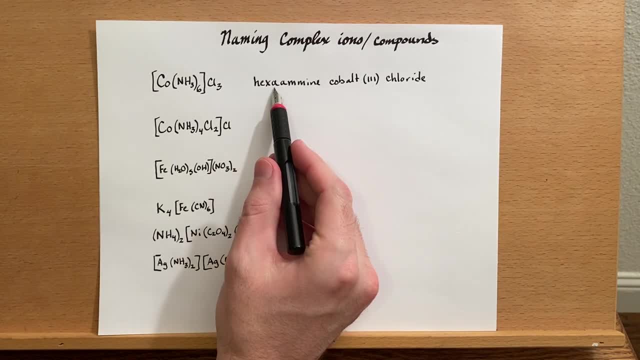 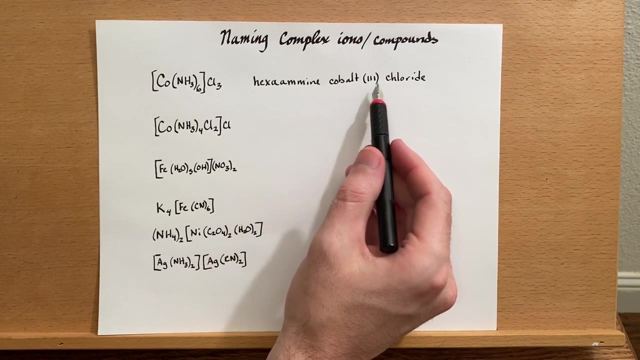 something good for non tropic 근 you. you see, this is a very, very common quadrant. so if you're talking about my, talked about when you, I wrote the term amineolly, that's the case. we say hexa amine, cobalt 3 and then chloride, because that's the 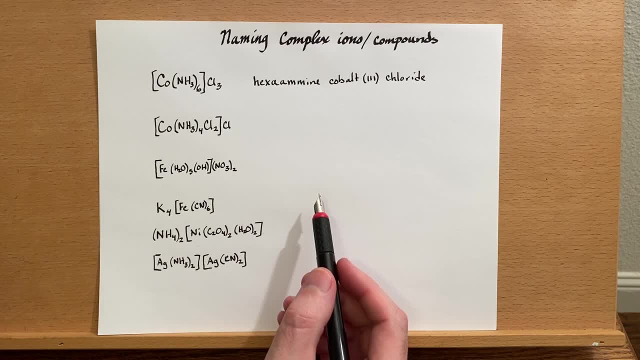 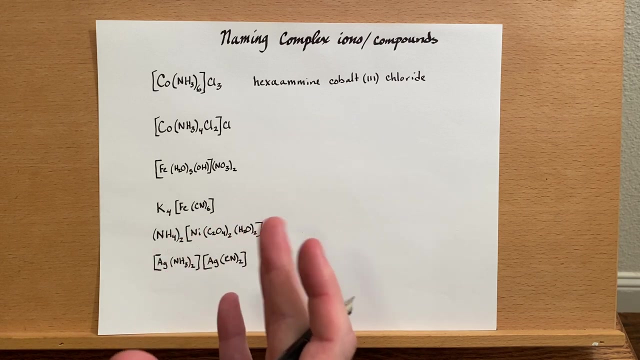 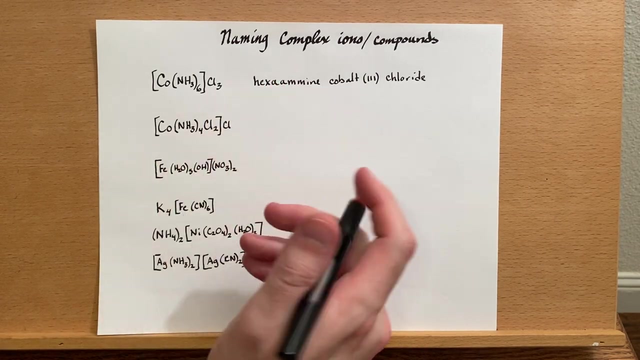 counter ion. now, I know it's a little odd to have that, because there are other times when we're naming like, for example, a inorganic compound that has you know four things in it and then an a coming up next, we would truncate that one of the A's, but in this case we don't and we keep it. 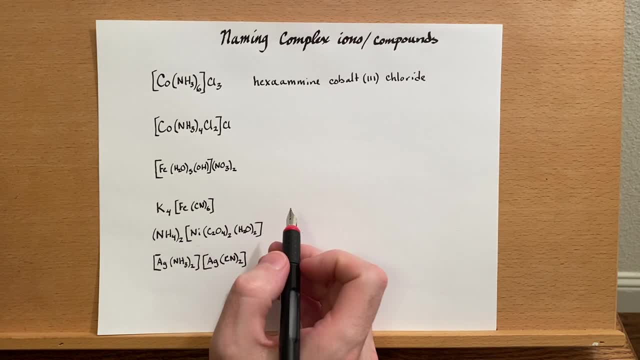 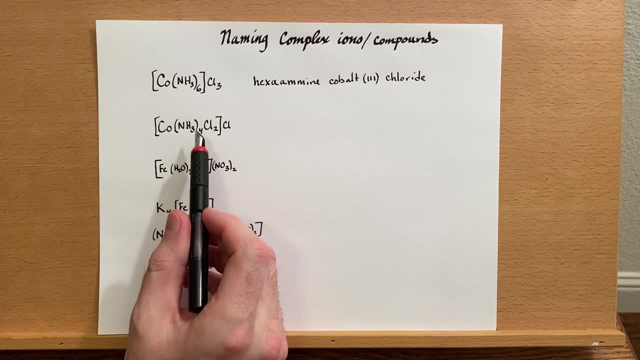 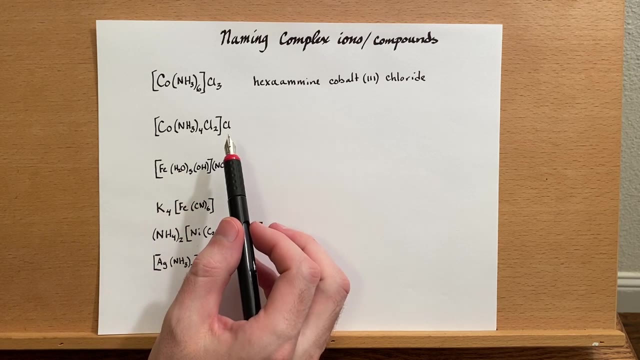 so just keep it in there. now this next one we have. we have two different ligands on the metal. now we're not going to worry about isomers, even though this one has two cis and trans isomers, but we'll ignore that part of the name for. 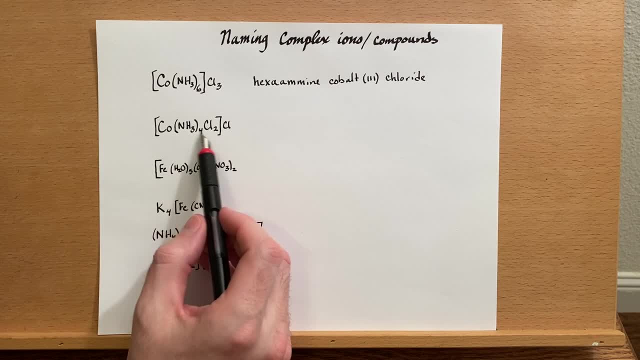 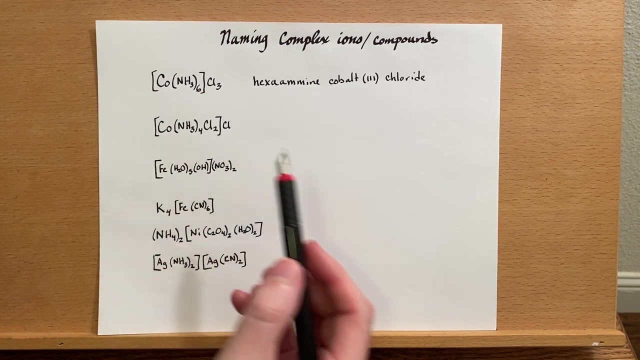 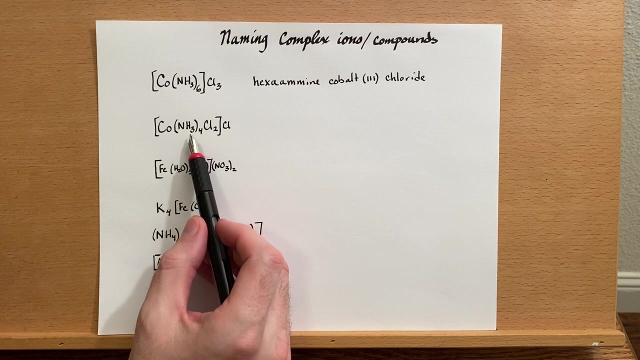 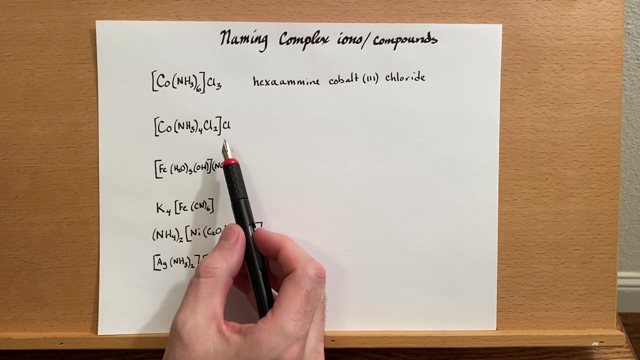 now and we need to know the rules for these two ligands. when, if you have here an a, has barresive love送ered to stored ligands and then this one has a single b, has barresive love doing the same stuff for the negative. negative and then for an: a has showed sin losingsa more min and has deduced a that one just want interest. needle those, sigma nucleus, chaloxanine, the, this one order they do they go in, do they just go in the way they're written? well, I try to. make it go in that way, but sometimes I might get it out of order. they actually just go in alphabetical order. so this is an amine, so that will go first. and this is chloro. it's not chloride. chloro when complex, when a ligand has very Joe Chales. 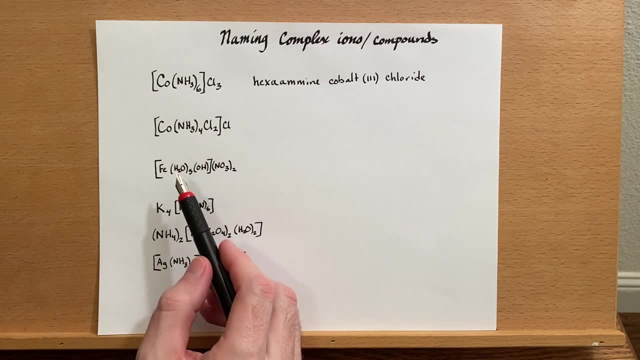 Hall and benchy. it's irreading. these are highsoping. these are not chloroplasma. cause d insyl doctor. but caustin has a negative charge. it ends in an O when it's a ligand, when it's bound to a metal. 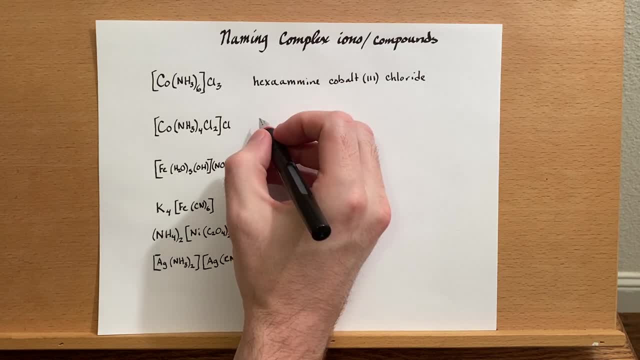 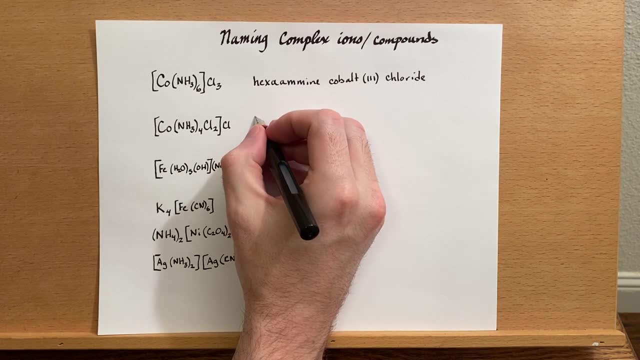 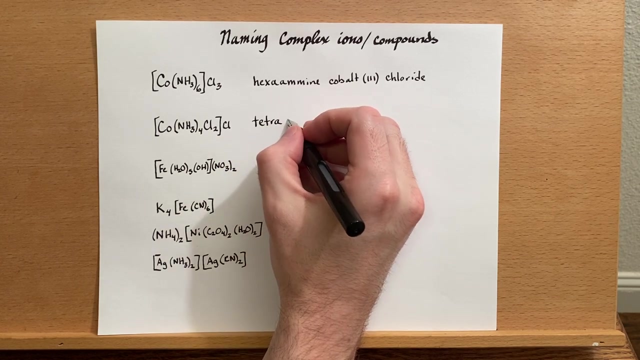 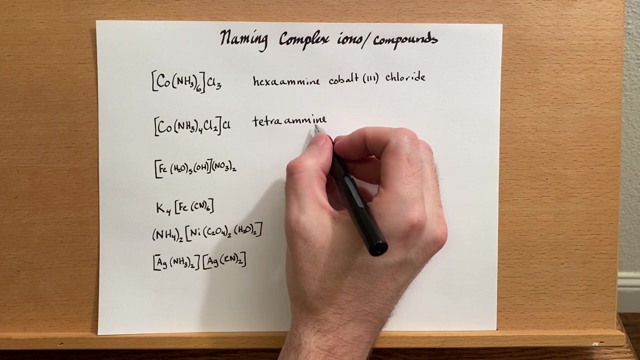 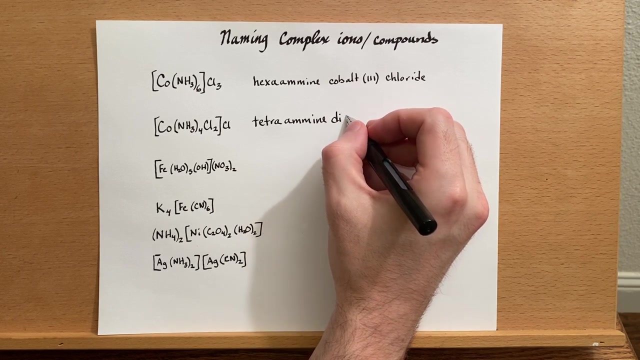 like this, So just keep that in mind. So the name for this would be tetraamine, because there's four amines. four is tetra. get the pen to work here. amine has two M's tetraamine and then two chlorides, so dichloro. 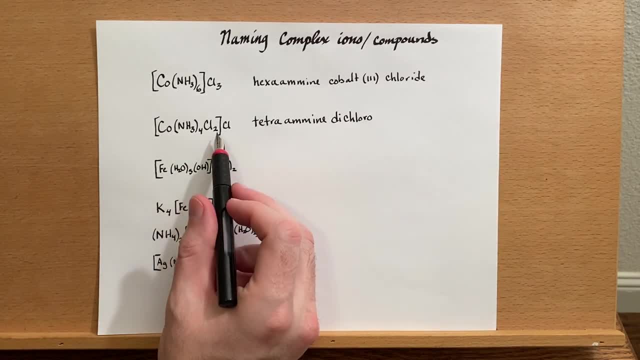 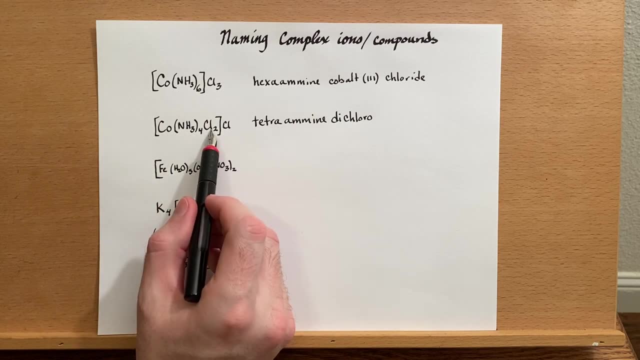 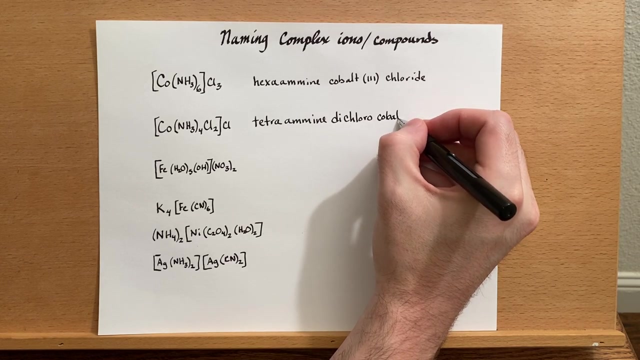 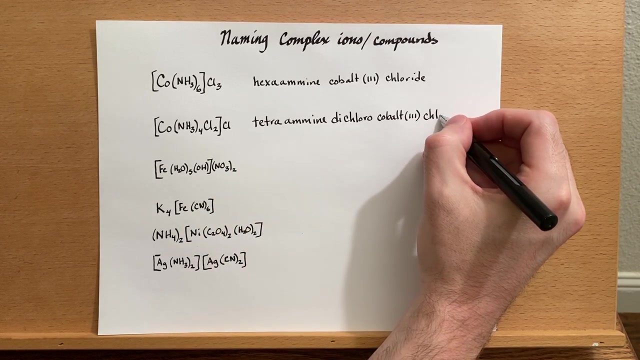 chloro ends in an O there, And then this is also cobalt-3.. So these are, These are negative. one charge, ligands, and so there's one, two, three negative charges. so this is cobalt-3. And then still chloride. 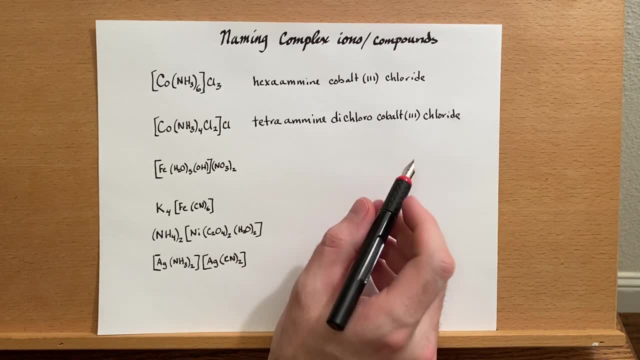 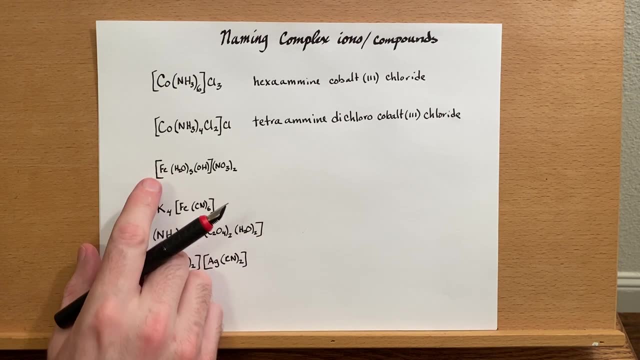 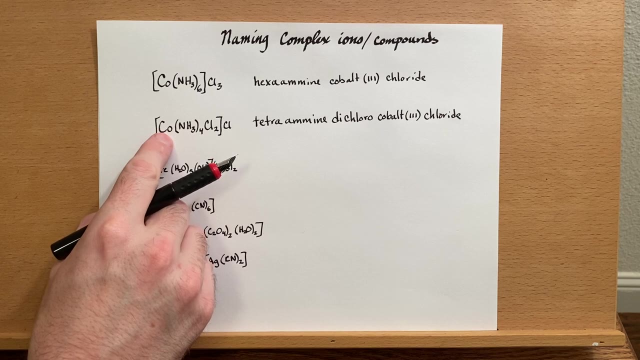 So just again, notice that this ends in an O when it's a ligand. All right, let's move down to this iron complex. Oh, and also notice that when we're writing the complex, we always write the metal first, but when we're writing the name, we always write it after the ligands. 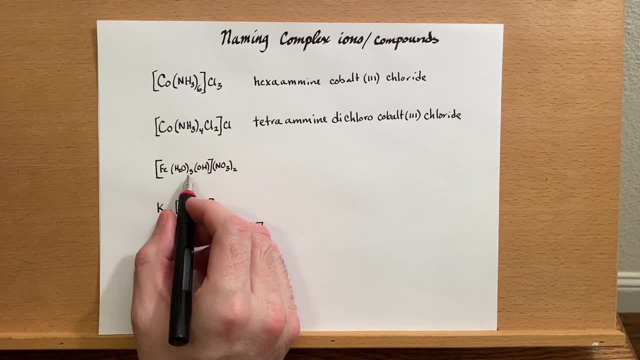 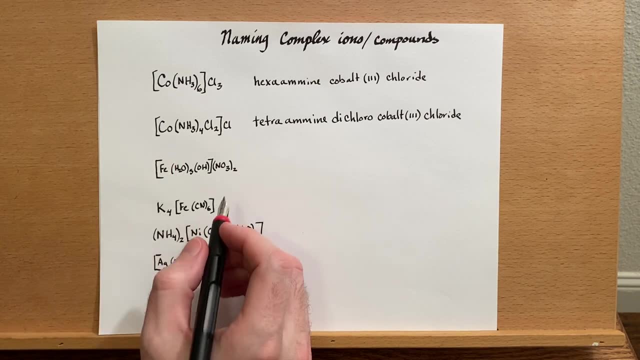 It's just how it's done. So here we have five waters as ligands and one hydroxide. Now, when water is a ligand, it's called hydroxide. It's just how it's done. So here we have five waters as ligands and one hydroxide. 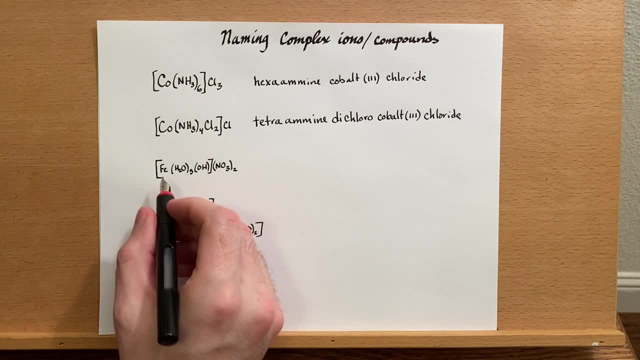 It's just how it's done. So here we have five waters as ligands and one hydroxide, And then still all of these have the same name. They just don't have the same name. They're called aqua, A-Q-U-A. 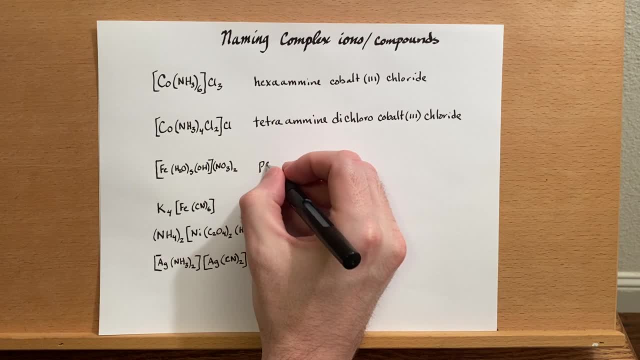 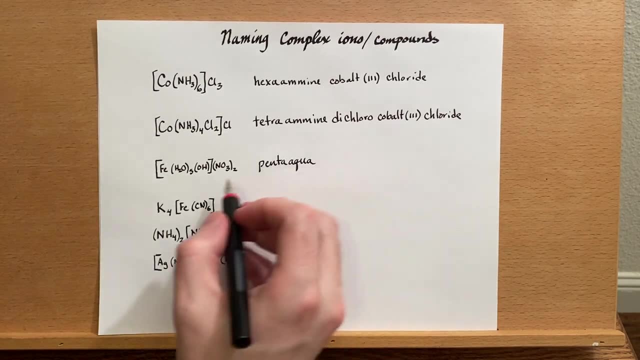 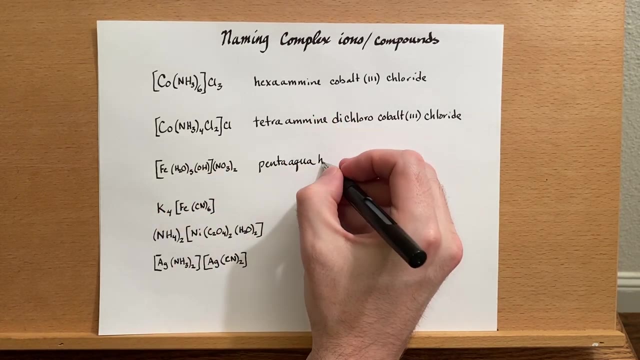 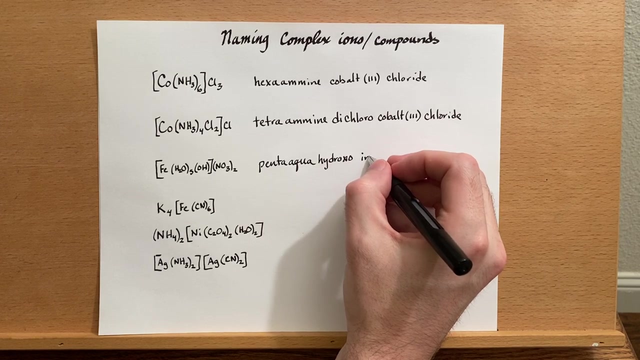 So this is penta-aqua, Penta-aqua and then hydroxide, but they have to end in an O, So this is called hydroxo, And then iron And then hydroxide. Attach the lid. Now what's the charge on the iron? I have a negative charge ligand here, hydroxide has one negative charge and I have two negative charged counter ions. so that's a plus three charge on the iron to balance out. So iron three and then nitrate, because that's the name of the counter ion. 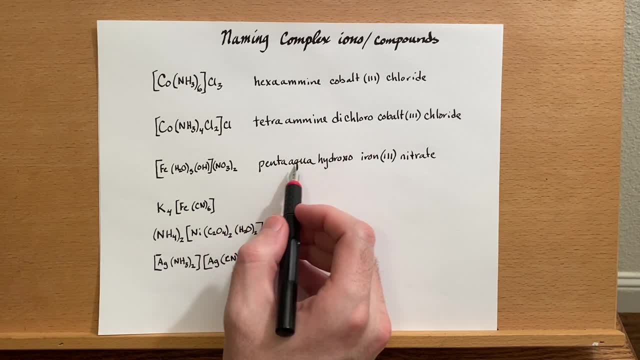 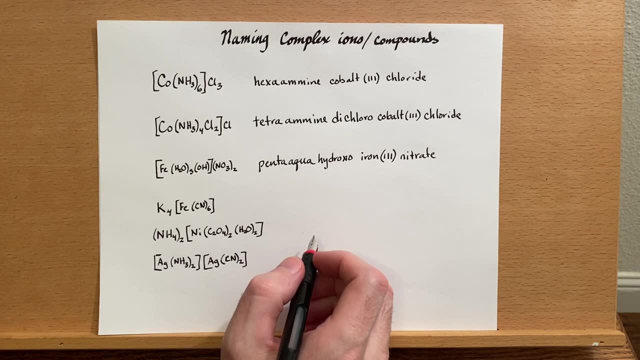 Okay, so remember alphabetical order. don't drop the A and you may have to look up some of these ligands, and you'll find it in most textbooks or online what the names of various ligands are, But you can probably guess what some of them are. 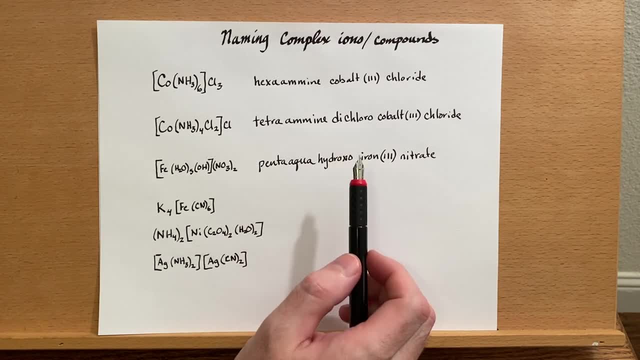 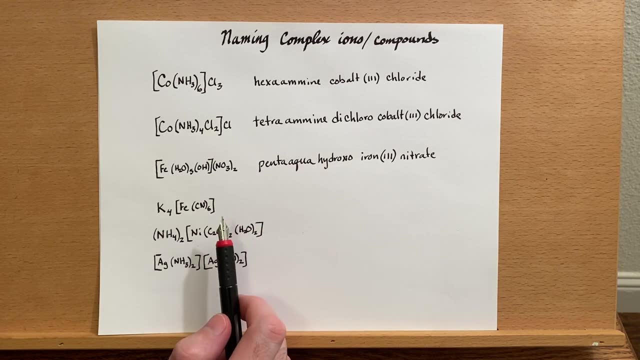 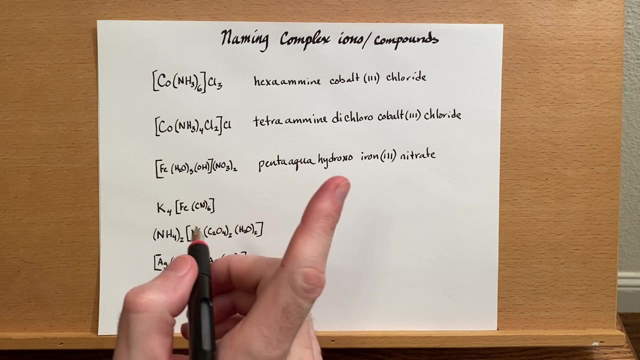 So, for example, if we had a bromine here instead of chlorine, you'd just call it bromo. If you had an iodine, you'd call it iodo. If you had a sulfate there, you'd call it sulfato ends in an O, because it's negatively. 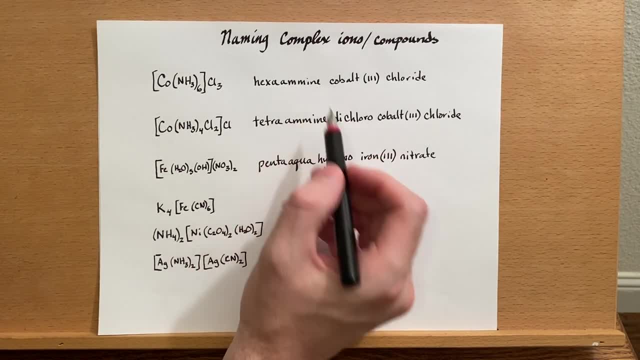 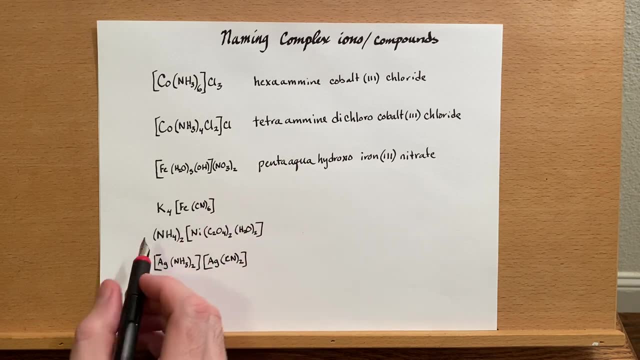 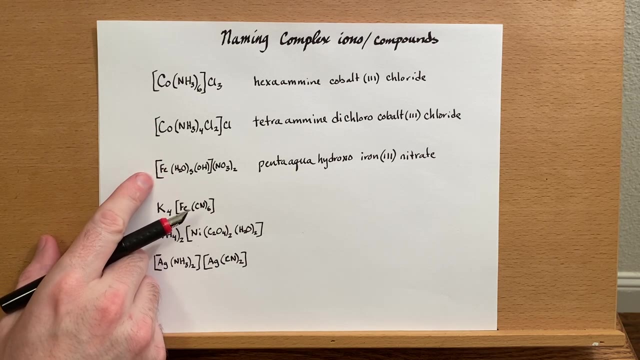 charged, These, the amines, the aqua, they don't end in an O, they're not negatively charged. that's why, All right, so we come down here Now. so far we've had the complex be the positive ion, but down here the complex is the negative. 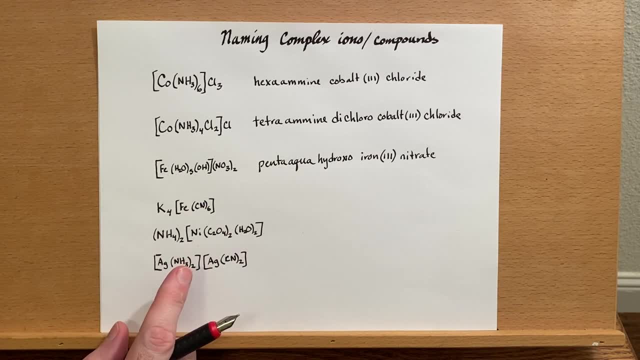 ion. Those get named slightly differently than when they're a positive ion. We need the complex to end in an A-T-E eight. So with the part that we definitely know, this is called potassium and when we have it in an ionic compound. 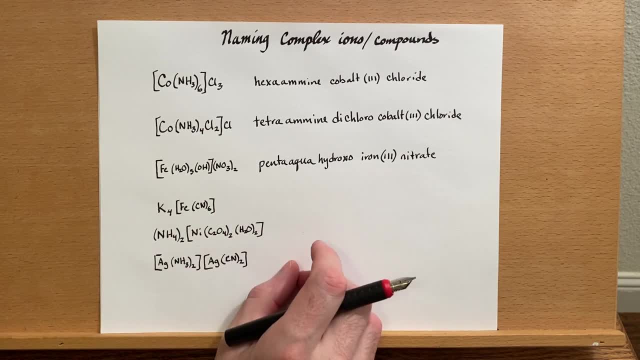 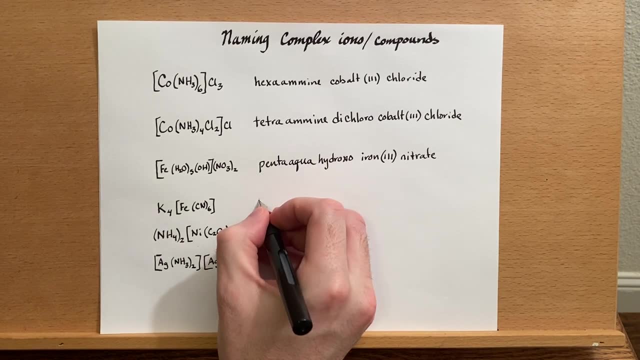 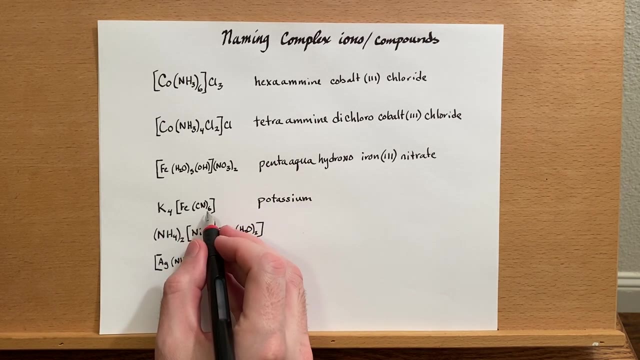 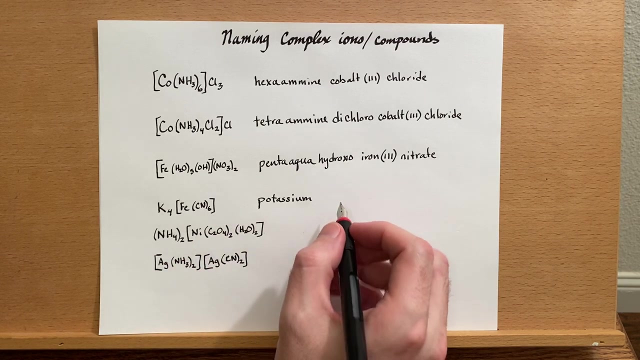 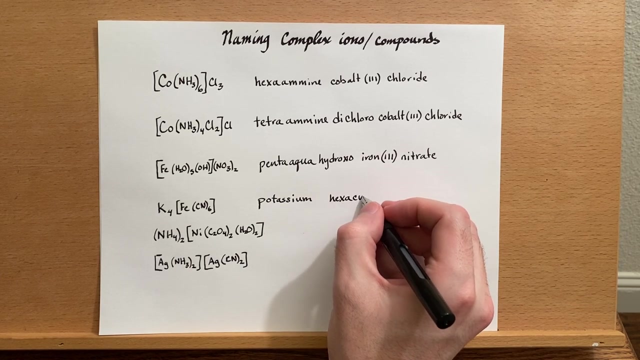 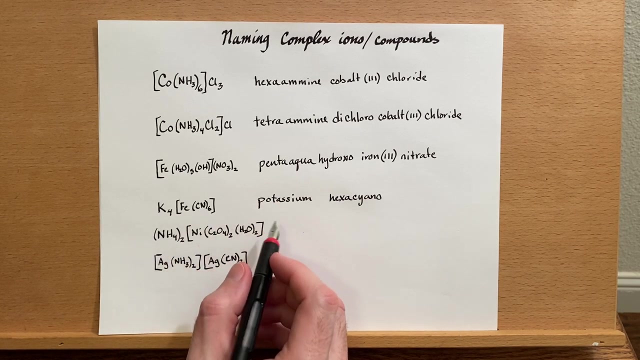 we just say potassium and then name of the negative charge ion, the anion second. so potassium. Now we need to name this Same story. ligands names come first. There's six, so hexacyano Cyano is the name for the cyanide ion when it's a ligand. 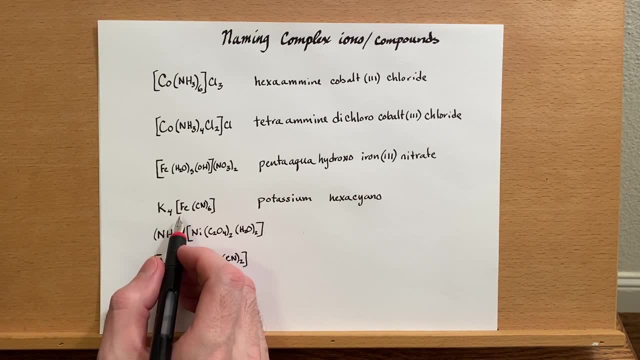 And then we come to the iron. Now we want it to be end in an A-T-E And iron eight. eh, it's just not as good. I suppose it could technically be correct, but there's a better name. We have to just look at the old style. 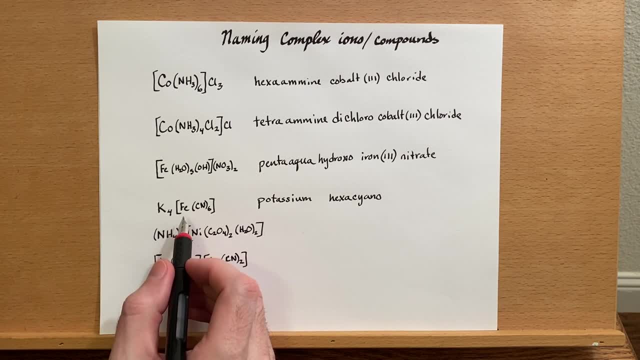 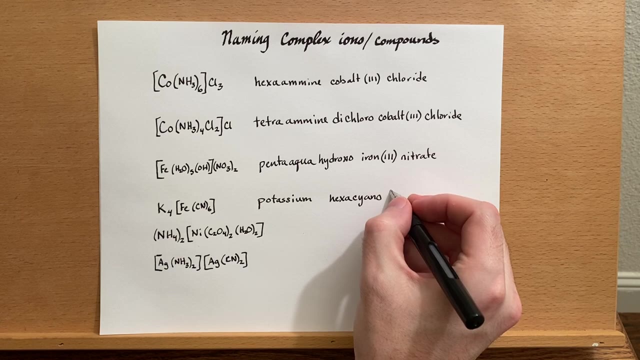 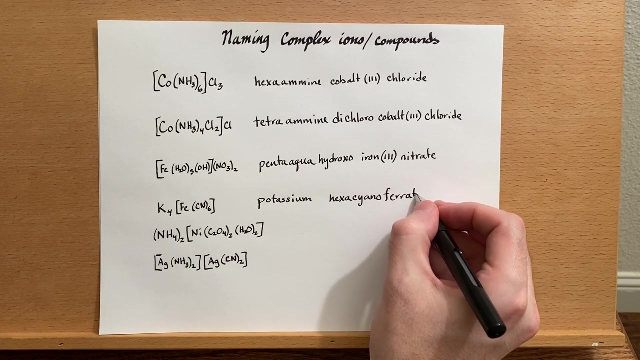 of naming compounds, then This is from ferrous, and we tend to use the name ferrate instead, the old style name, because it sounds a little bit better. There may be other reasons, but to me So ferrate. And then we have to evaluate the charge on it. 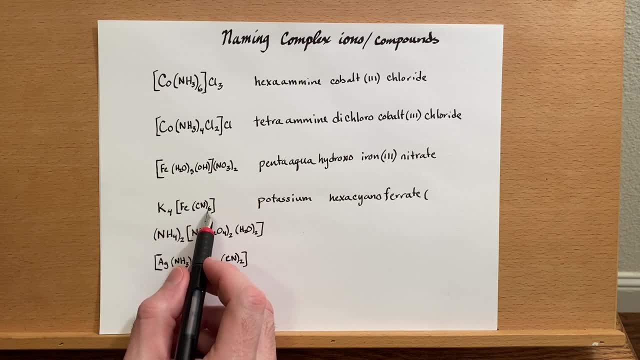 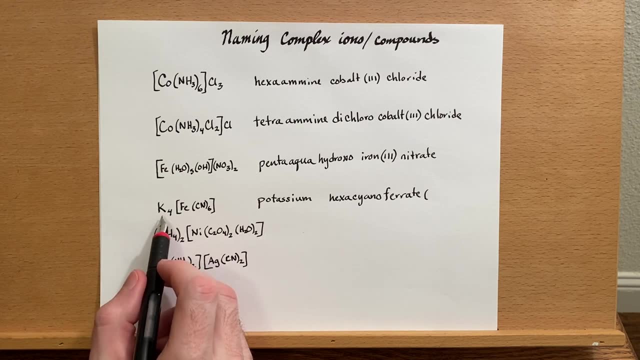 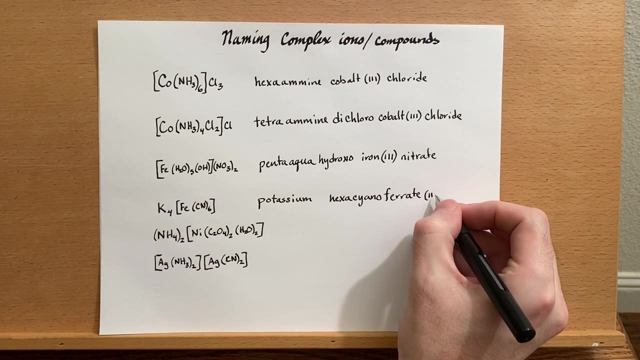 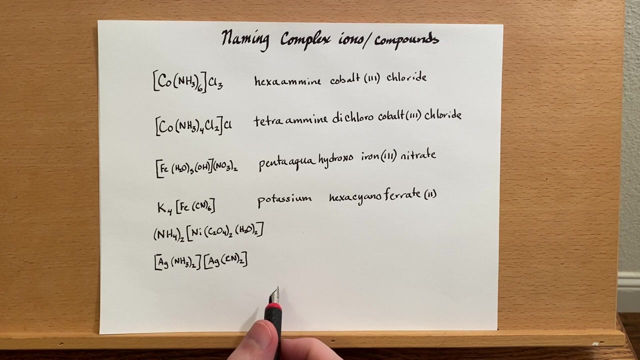 So cyanide is a negatively charged ligand. There's six negative charges. Potassium is a plus one charge on it. So that leaves us with two positive charges. for the iron, so ferrate two. so potassium, hexacyano, ferrate two. all right, I have another one down here that also contains: 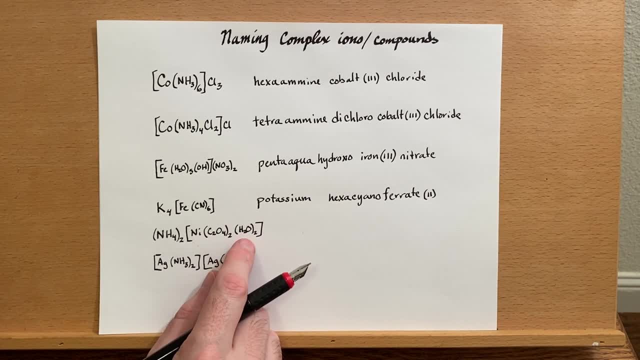 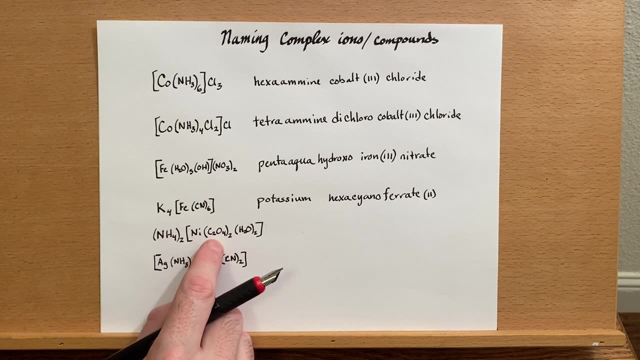 a negatively charged complex, but we have something else with it. that's this: we have the oxalate ligand. now, oxalate ligands are by dentate, they're chelating ligands. they attach in more than one spot, they attach in two spots. so these 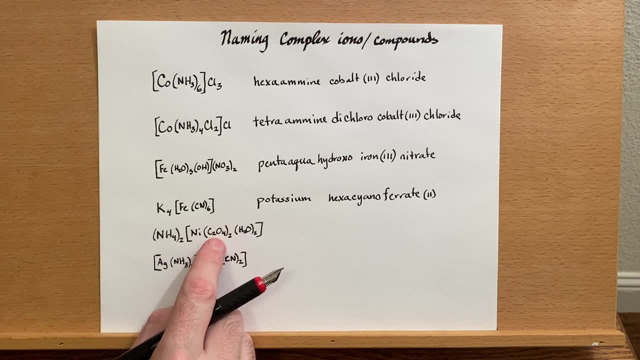 get their own special naming system. instead of die and try and tetra and all of that, they get this tris and tetra kiss. I'm sure there are more beyond that, but generally speaking you won't encounter ions that have so many on there because a chelating 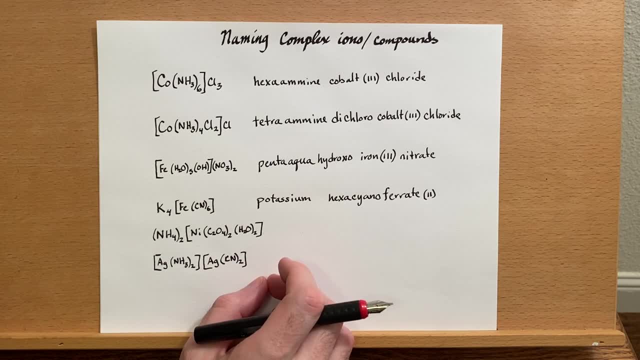 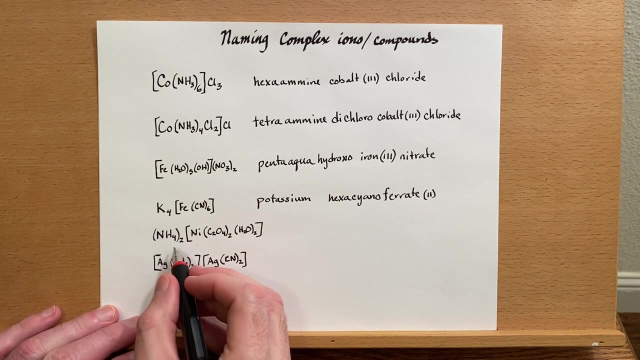 ligand bonding to an octahedral complex. at a minimum you're going to attach at two points. octahedral complexes have six attachment points, so really you're going to encounter this and tris ligands more than tetra, kiss and beyond betterThis after every. 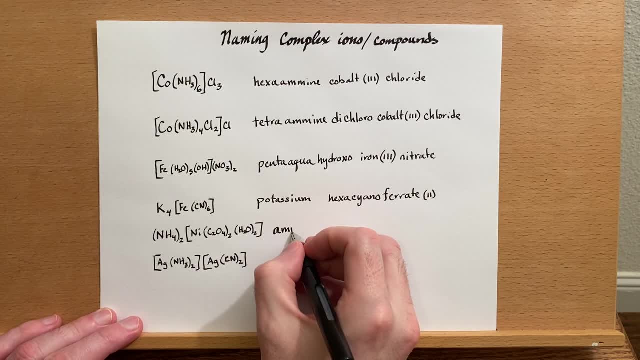 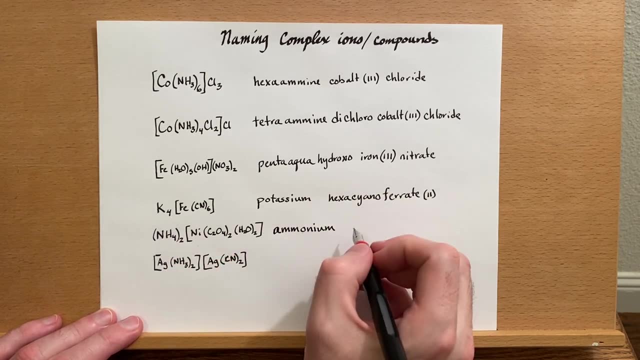 sea part was Burke czar, about two hours, and there was no have the initial step down for the next stage ofентов up这是 just because of space requirements, alright, so let's go ahead and name this. so we start with the positively charged ion first, and that's ammonium, six steps after still being in 알ne. 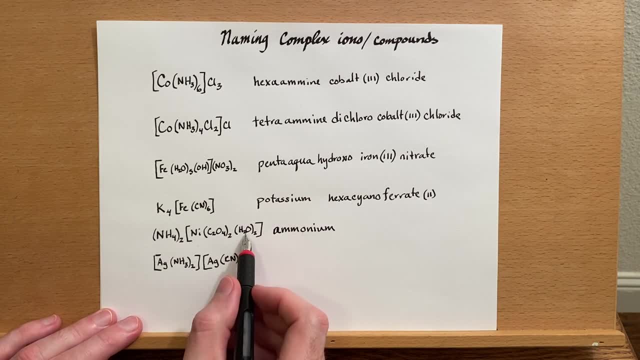 order. so this is water ligands right here. and then there's oxalate. water has is called aqua and this is oxalate. so that starts with an A, that starts with an O. this one should be named first. so it's dye aqua, because there's two of. 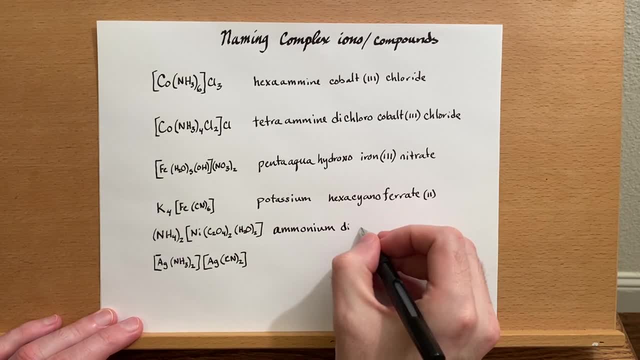 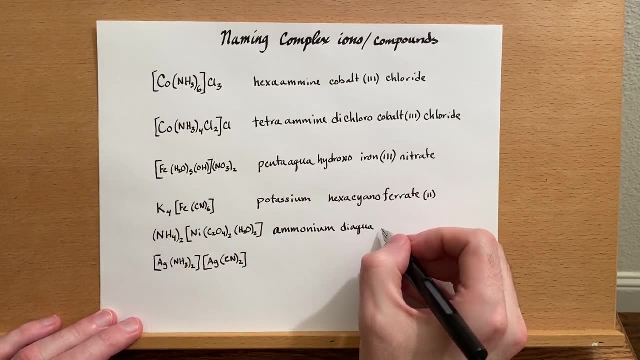 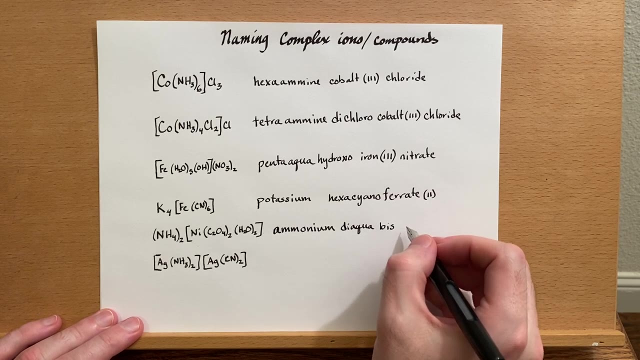 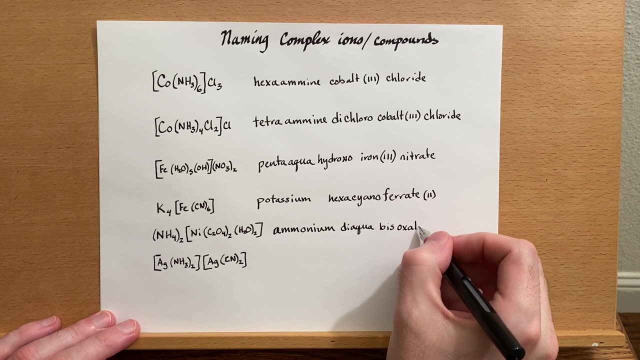 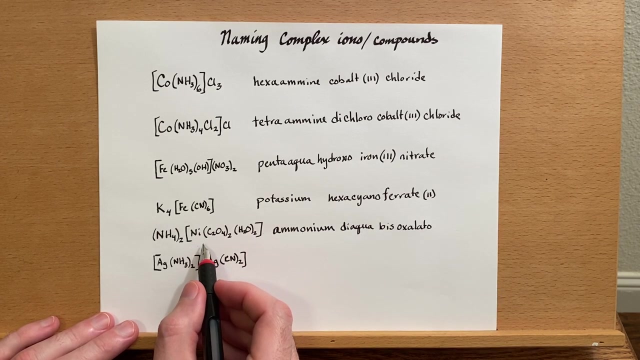 them. and then there are two oxalates, but it's chelating, so we call it bis, bis oxalato, because again it's negatively charged. and then we come to the next part of the process, which is the chelating of the nickel, and it needs to end in an eight and there's not a very nice way, like the. 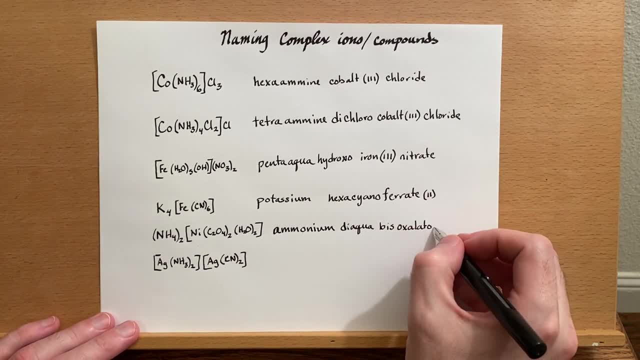 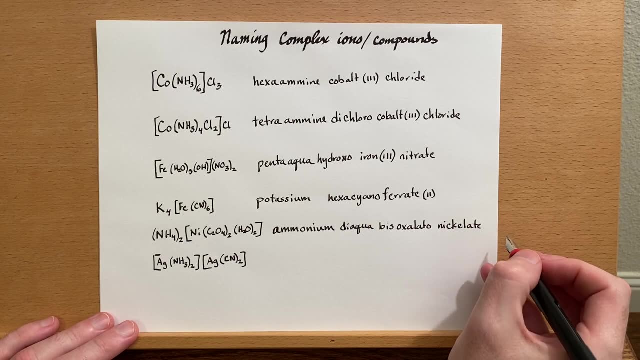 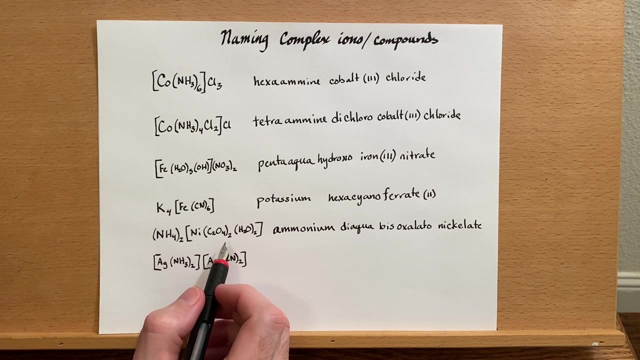 iron to go with, so it's just nickel eight and then the charge on the nickel. let's see here: oxalate is a negative two charge ligand, so there's a negative four right here, but these are two charge ligands, so there's a negative two charge ligand, so there's a negative four right here, but these are. 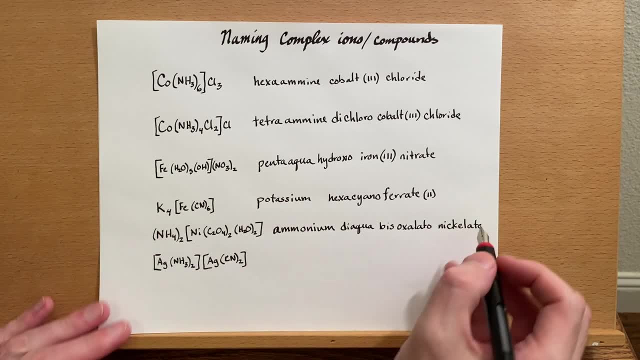 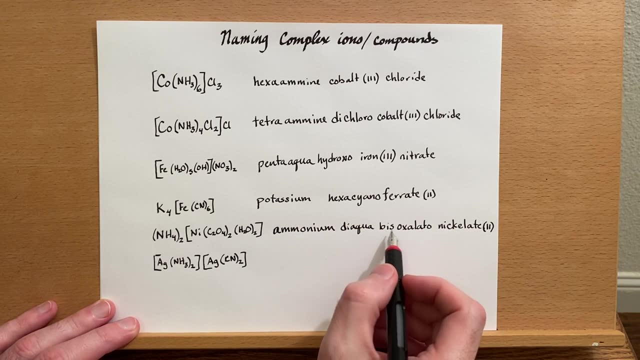 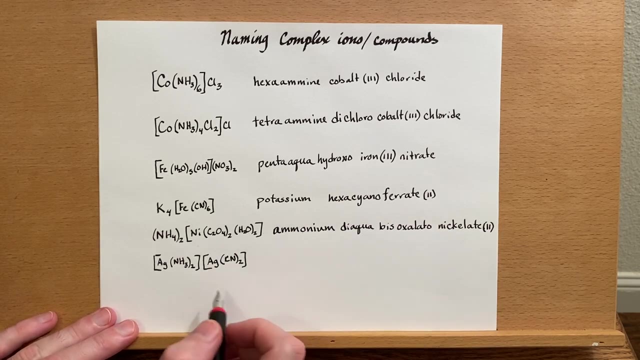 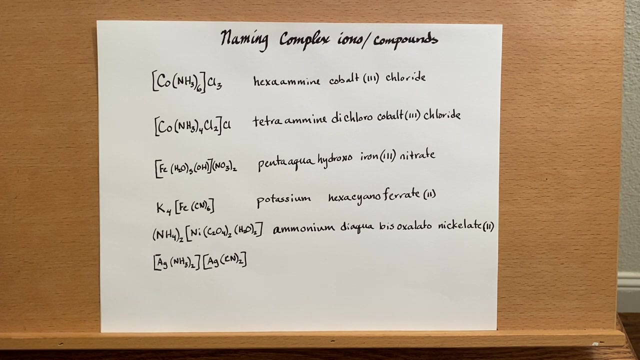 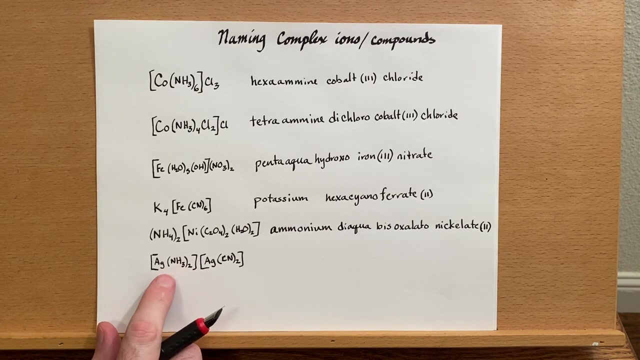 plus two. so this one must be plus two. so nickel: two. so ammonium dye, aqua bis oxalato, nickel eight two. now we come to an interesting case down here. it is possible to have both of the ions be coordination compounds. no rule against it, and so in this case we have a silver positive ion, and in this case we have a. 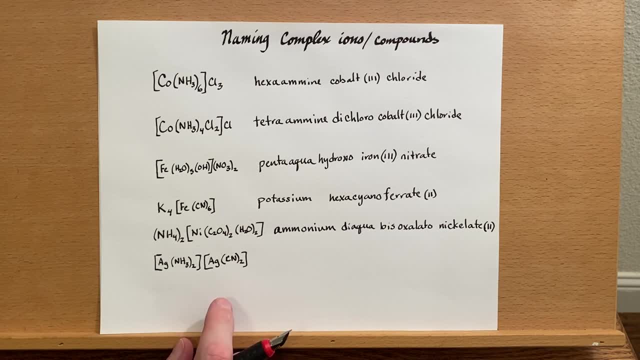 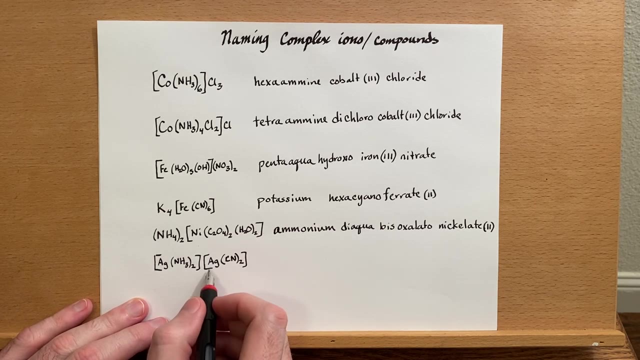 silver negative ion. well, what does that do to the name? well, again, we just name the positively charged ion first, then we name the negatively charged ion, and you'll notice that we'll have to change this to be an eight ATE, because it's negatively charged and over here we won't have to do that. so this is a. 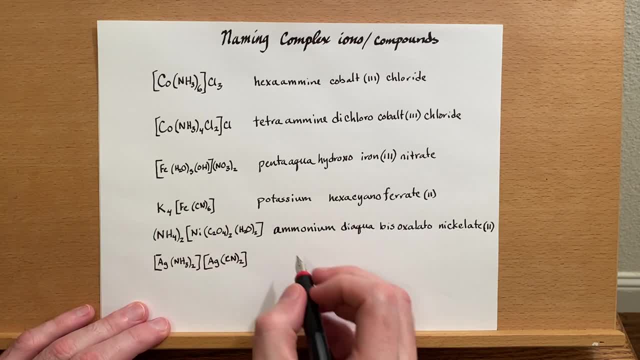 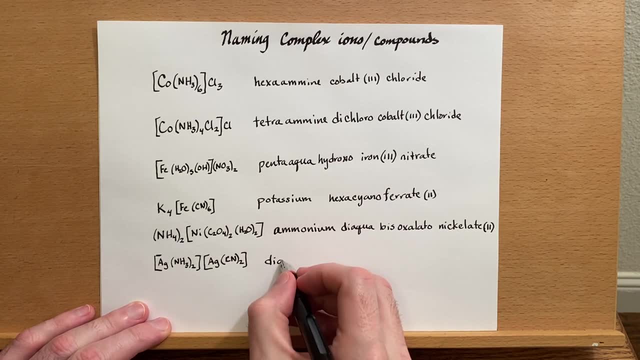 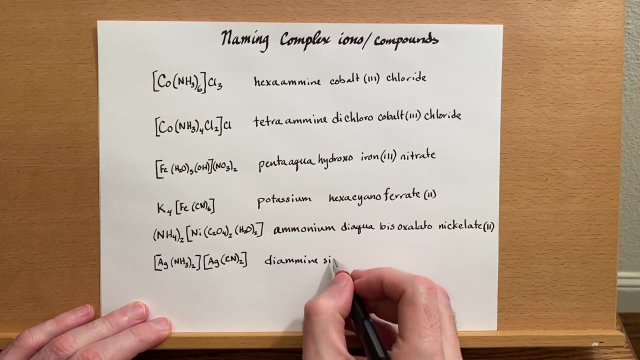 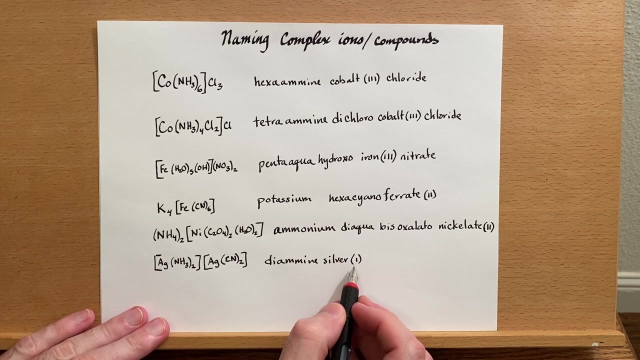 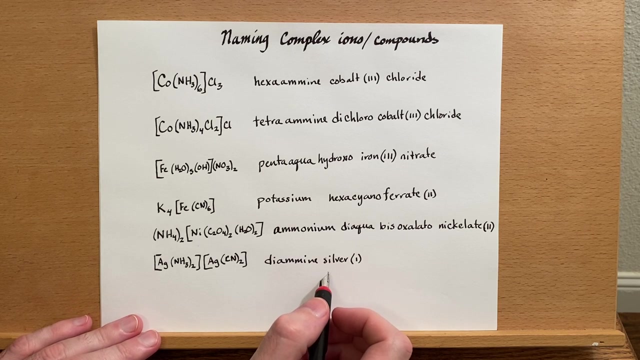 neutral ligand. so if we look here, we'll have diamine and then silver one. you might ask yourself why did he put a 1 there when silver is supposedly always plus one? Well, it turns out in general chemistry. a lot of times people tend to lie to you, whether they like to or not. 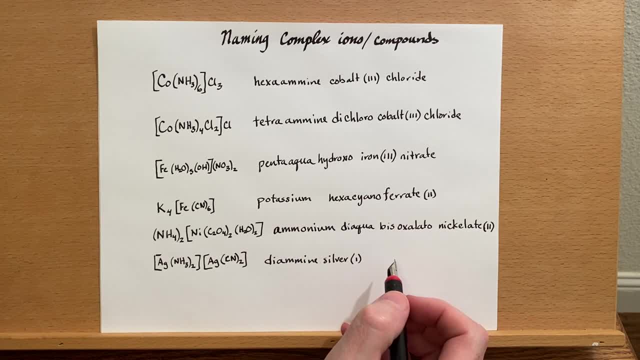 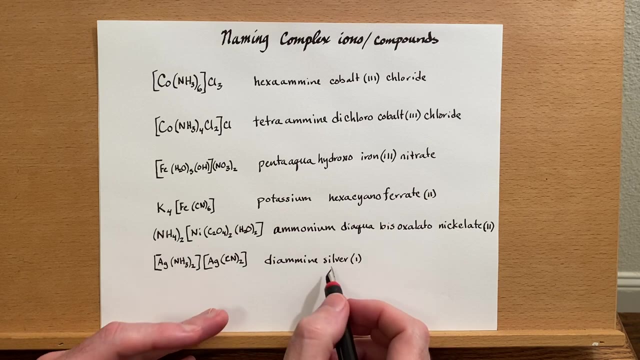 I don't think we actually like doing that, but there are cases when silver has a charge that's different than one. It's really rare, but it could come up when we're talking about complex ions. It doesn't in this case, but it doesn't hurt to write the charge for coordination compound. 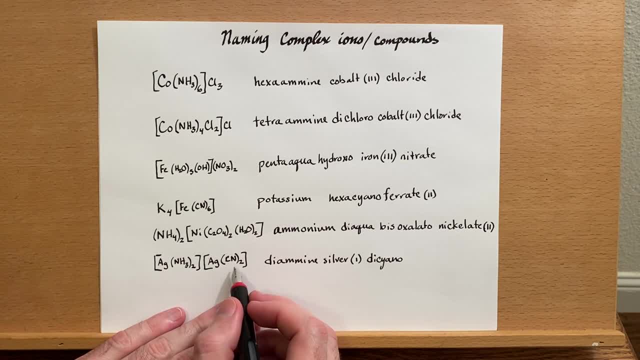 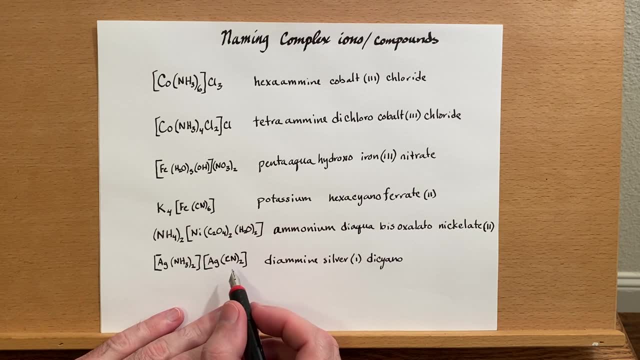 Alright, so there's two cyanide groups on here. Those have a negative one charge, and then we come to the silver. What do we call it? Well, the old style name for that is Argentum, and typically when we have a choice, when 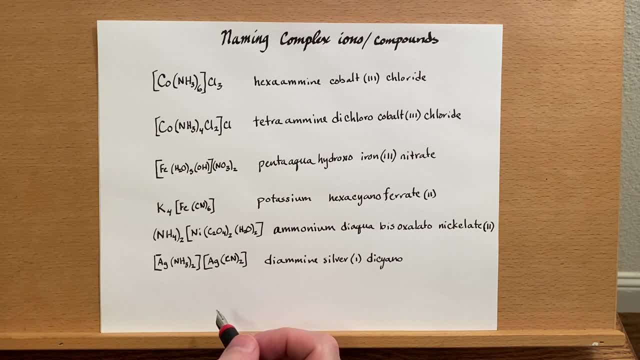 adding an A-T-E to the name. a lot of times the older style name has a more pleasing sound. You know, iron 8 just doesn't sound as good as ferrate and in this case silver 8 wouldn't sound very good. But Argentate doesn't sound as good as ferrate. 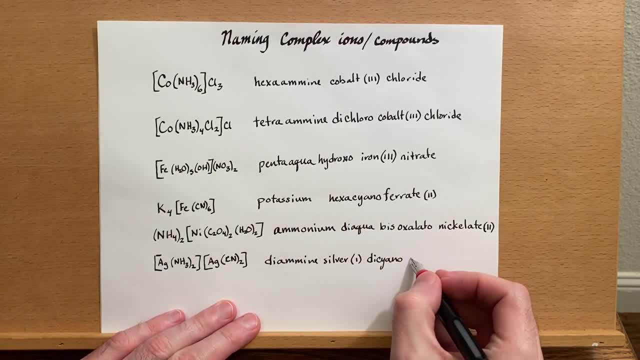 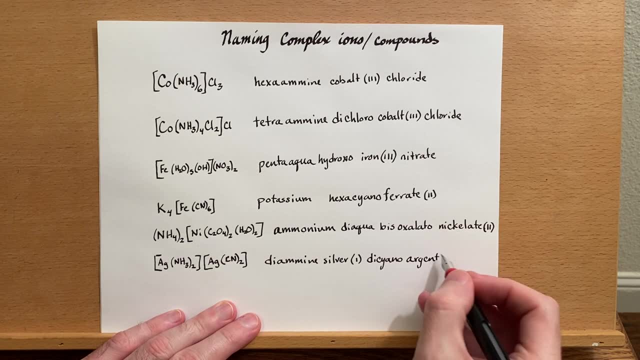 But Argentate doesn't sound as good as ferrate. But Argentate doesn't sound as good as ferrate, But Argentate does. so we call it that, And that similarly also has a plus one charge on it, So Argentate. 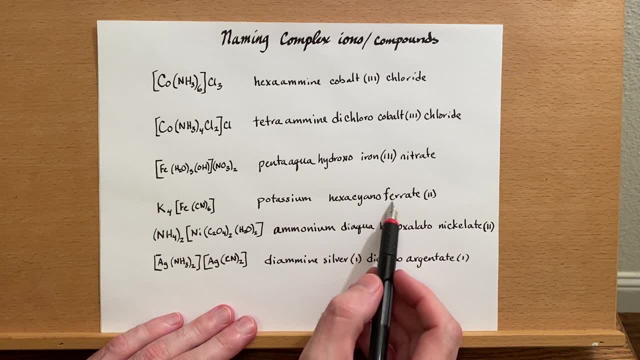 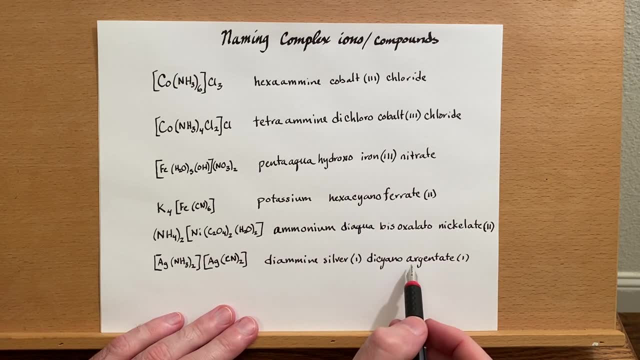 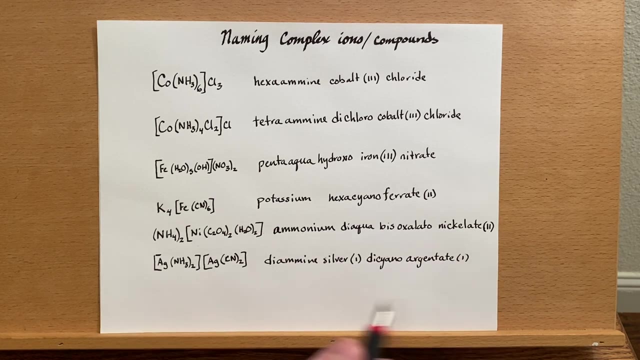 And now you may know where the iron name comes from and you may know where, or the symbol F-E, And you may also now notice where A-G for silver comes from Argentate. So that's just a little bit about naming complexes. 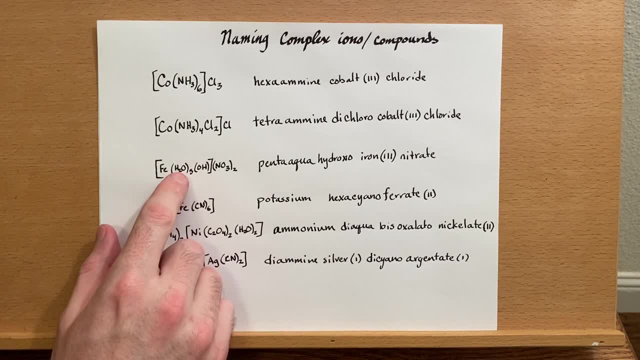 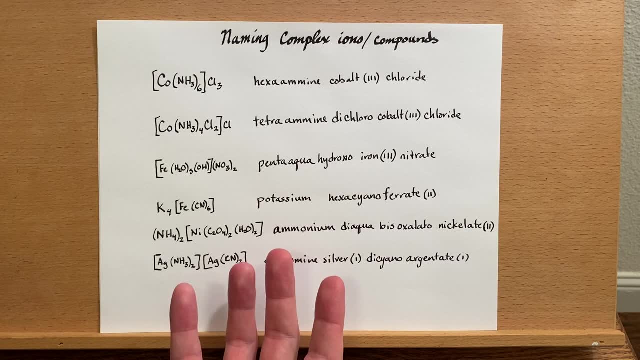 It's possible to have lots of different ligands on a complex, As you can see here. we only had two on here, but I could have added a few more. We only had two on here, but I could have added a few more. We only had two on here, but I could have added a few more. 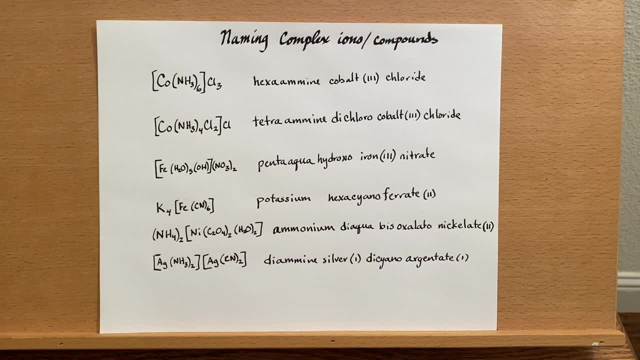 More on, And it's just a matter of making sure they're in alphabetical order and denoting how many of them there are There.